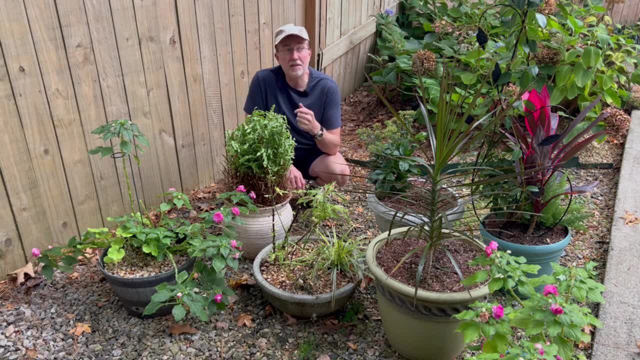 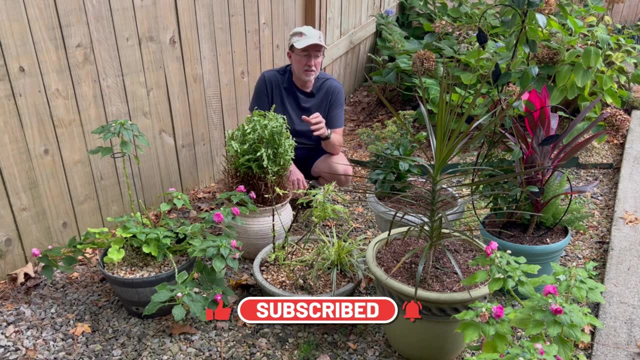 So, guys, it is that time of year where we start bringing our potted plants into our homes, basements, garages and greenhouses, And a lot of times we bring in a colony of ants without even realizing it, And there's a couple of things that you can do that will absolutely stop that from. 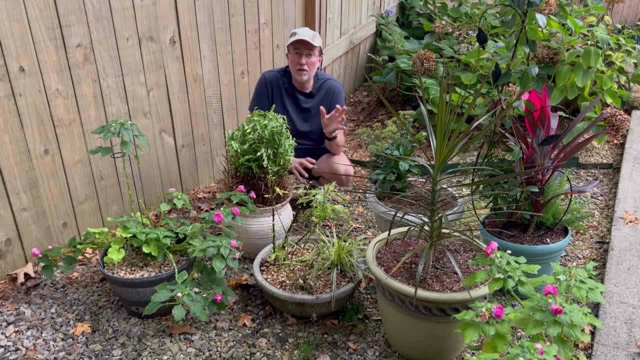 invading your home, anywhere that your living space is, and you don't have to worry about it taking over your pantry at some point. So I'm going to get these to the greenhouse and I'll show you the most effective way, the two most effective ways I know, to stop the ants from. 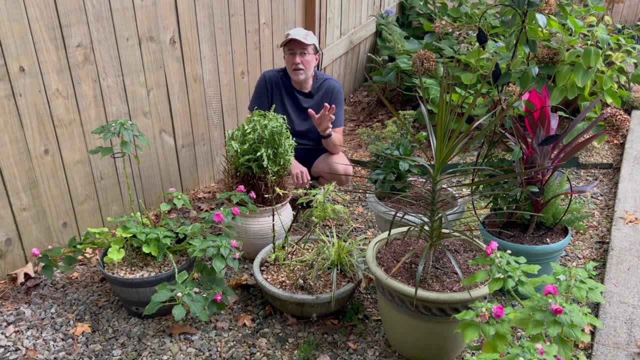 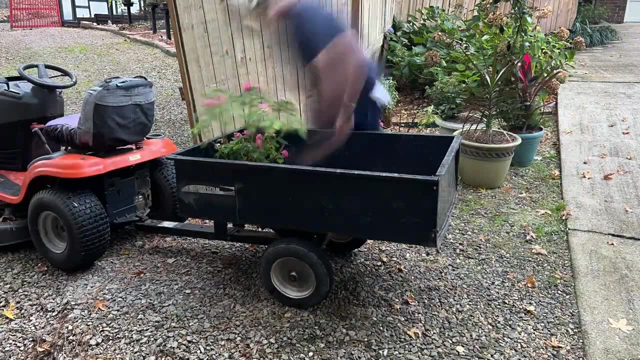 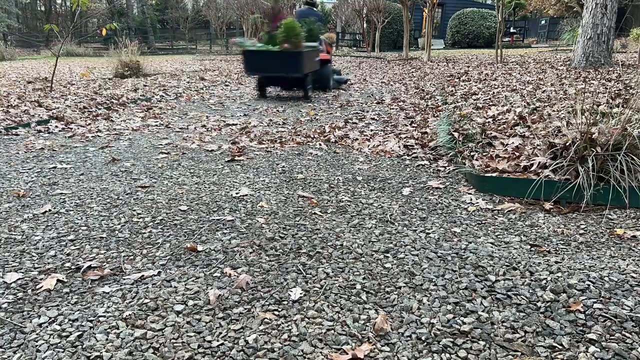 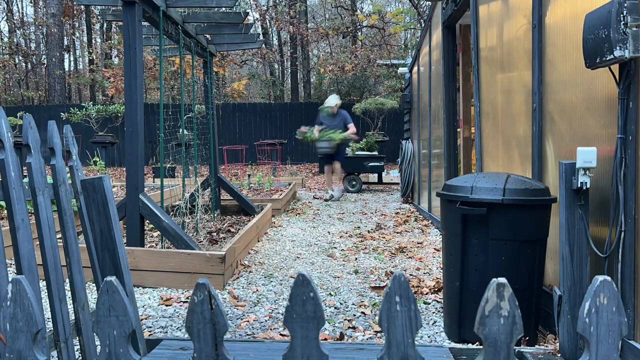 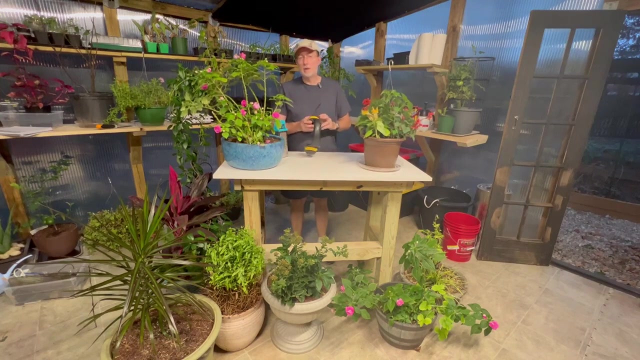 living in your potted plants and a lot of ways that are not effective, but there's a lot of stories behind them that they do work, but there's little evidence that they do So, guys, as you can see, this is only one corner of the greenhouse and it's still. 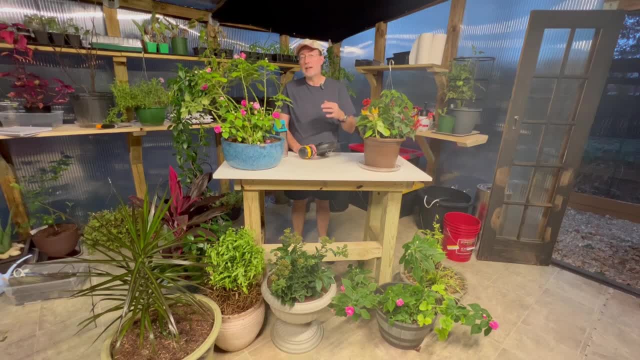 only partially filled By the time all the bonsai come inside. I'm going to barely have walking room, But what I wanted to show you today is something very critical to bringing plants inside your home. when it comes to ants, You want to prevent a total infestation, because they may go. 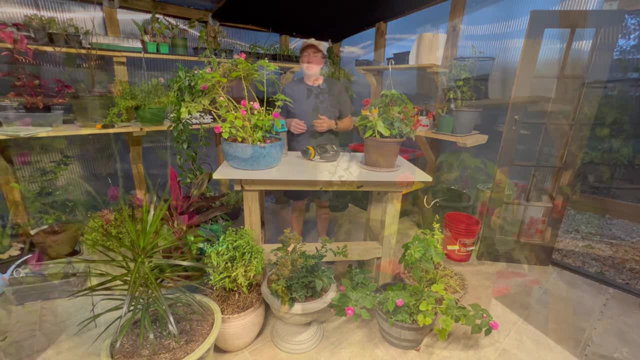 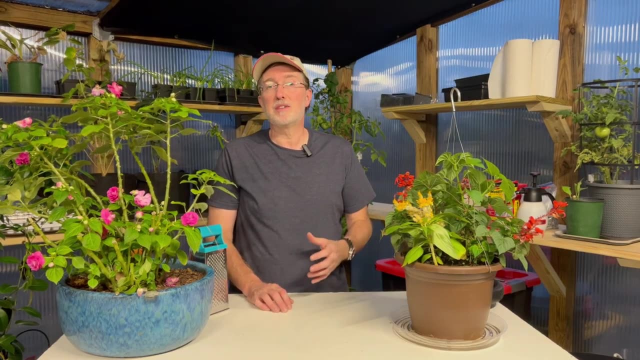 from your plant to your pantry, and then you've got an even bigger problem. So, guys, I'm hoping the sound of the rain on the roof of the greenhouse isn't drowning me out. I had to shut the doors Because the ever-present sound of leaf blowers throughout the entire neighborhood is echoing. 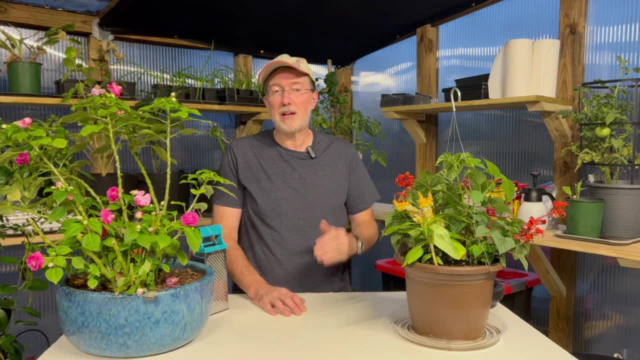 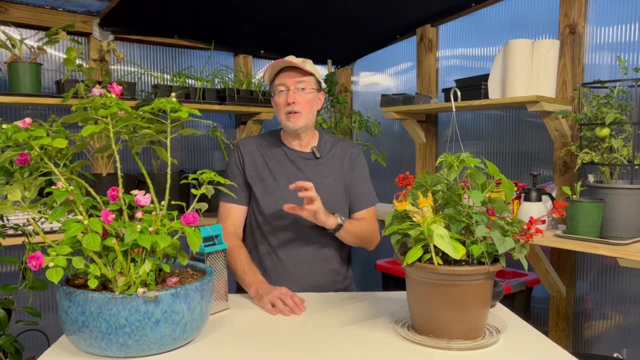 around the entire yard, So I think my microphone will cancel that out, But anyways, what I'm talking about today is two specific ways that absolutely work to keep ants from coming in your house from your potted plants, And these two products are completely safe, completely organic. 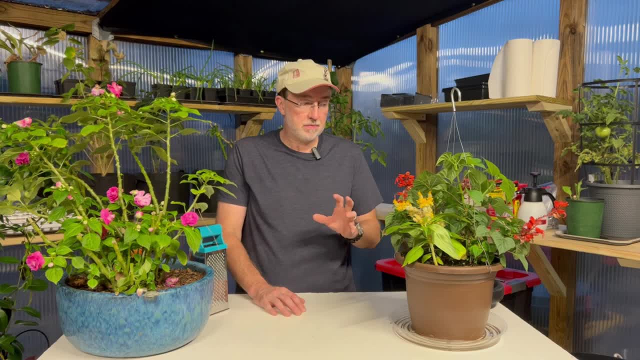 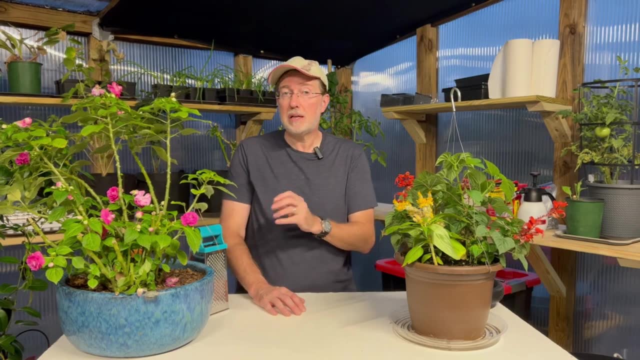 And one of them we actually consume. The other can be consumed, but it's very rare that it is. But those two products will absolutely work to, one to repair and the other to kill. Now, since I have a very large number of houseplants thanks to my wife, 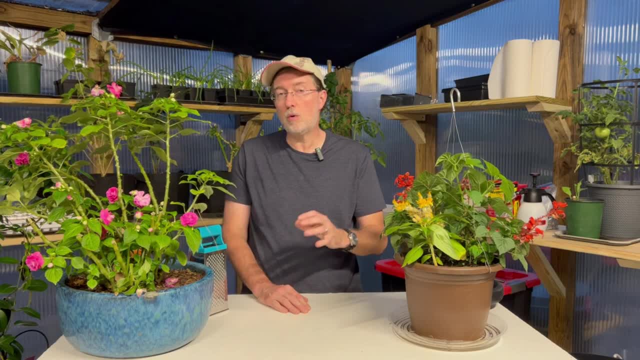 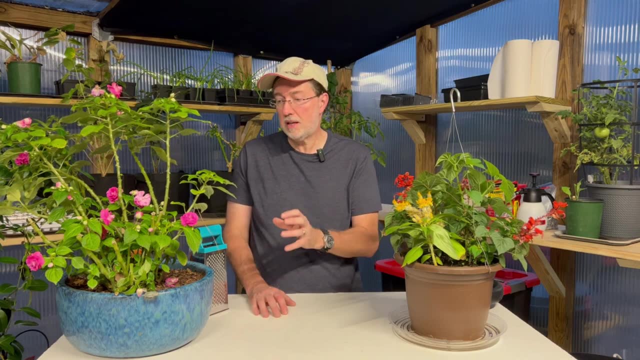 I also have even more bonsai in pots and I'm always dealing with ants in the yard, So it's an ever-present problem in potted plants. because they have just the right conditions for ants to take up residence: Perfect amount of moisture. They can go in and out of the pot. 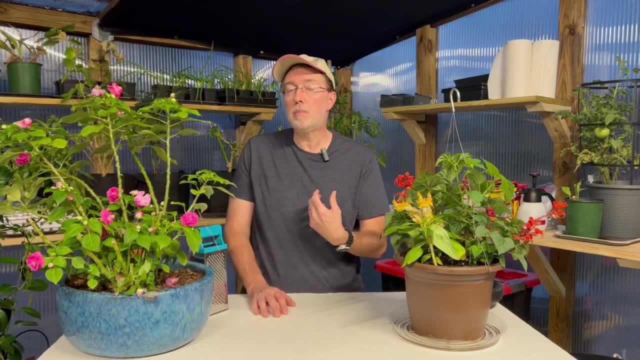 to go get food sources And sometimes there may be aphids on the potted plants and that can be a food source in itself. So the first product I've used in the potted plant is a plant that I've used in the potted plant And it's a plant that I've used in the 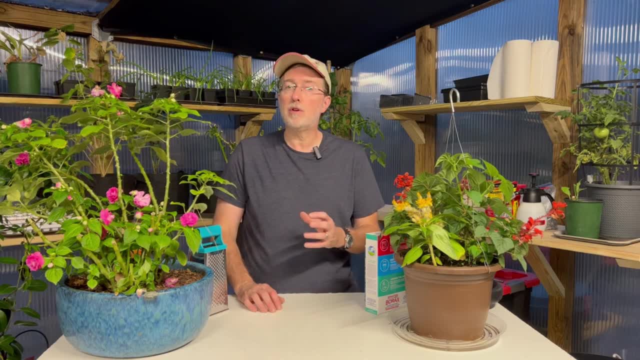 past that, one of the first things I actually tried was used coffee grounds unflavored, And that had very little effect on the ants. Now, maybe on certain varieties of ants it may repel them, but it's certainly not going to kill them, And for me personally it just didn't have much of. 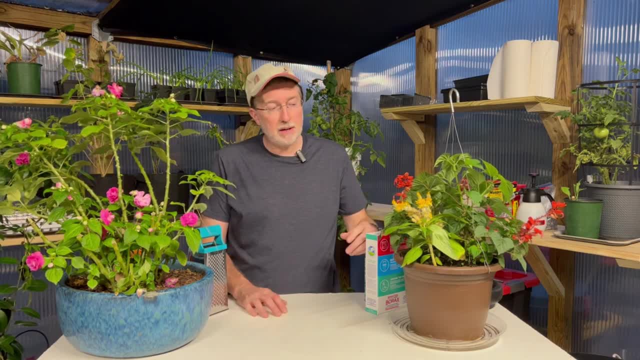 an effect. Now some people recommend cornstarch. I have tried that as well in the past. I put it around the perimeter of the pots and I would only see ants go up to it, slow down for a second and then walk right across it, And it had little to absolutely no effect on all. 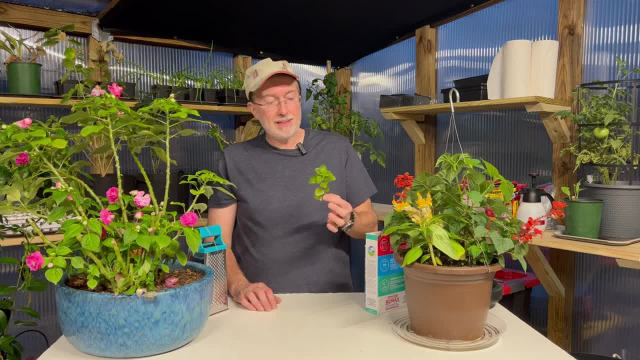 the varieties of ants I have living in my yard. Now, another product that a lot of people say works great is peppermint, or the different varieties of mint leaves, dried or fresh, And I found that, no, it didn't have any effect at all. Matter of fact, in one of my four by eight, 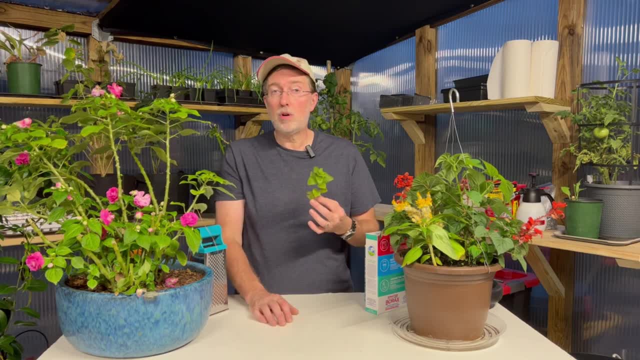 beds. I actually had a small ant bed forming in the corner of that bed, right next to the peppermint leaves or the mint leaves. This particular variety, I believe, is chocolate mint, but it's just a fancy name to just mint. But anyways, mint, whether dried or an actual, 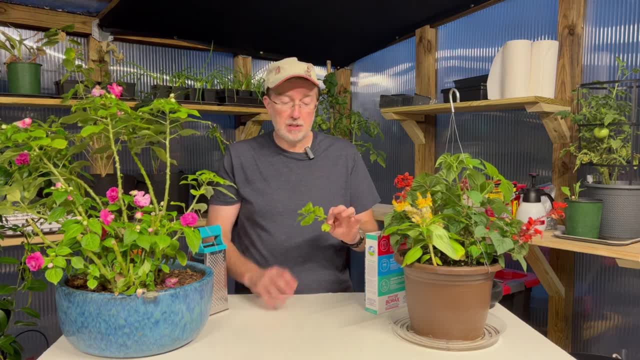 leaf sprinkled around it. it doesn't have any effect. And I found that, no, it didn't have any effect at all. Matter of fact, in one of my four by eight beds I actually had a small ant bed formed in the corner of that bed, right next to the peppermint leaves or the mint leaves, And I found that? no, it didn't have any effect at all. Matter of fact, in one of my four by eight beds, it doesn't have any effect at all. Matter of fact, in one of my four by eight beds, it doesn't have any. 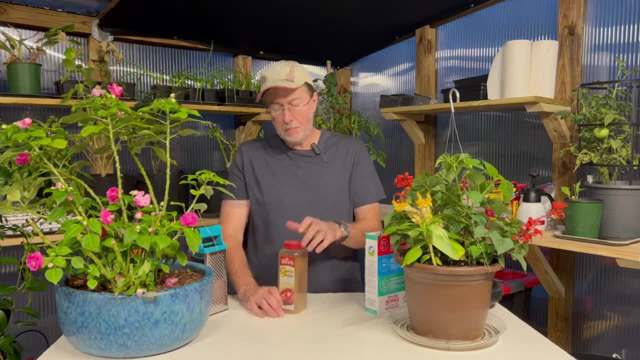 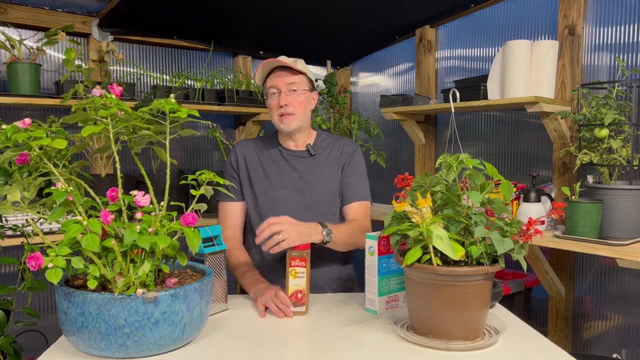 effect And, like I said, they actually took up residence right next to it. Now some people have also talked about using black pepper or dried pepper or cayenne pepper Also. I've tried that around the pots and it had very limited effect. Maybe on certain varieties of ants it might have. 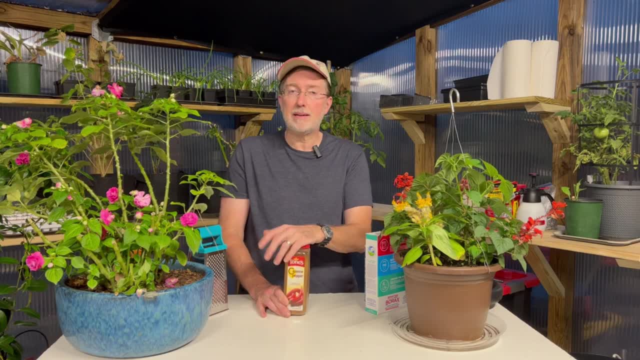 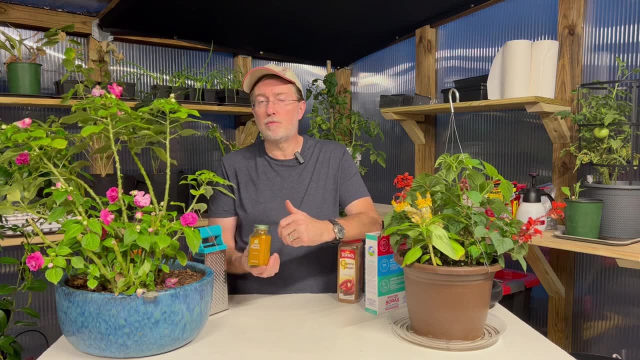 some effect, but as far as from my personal experience, no, it's had none at all. Now, Tumeric is kind of an interesting thing that I've tried because I did see some ants would avoid it. But eventually the ants would cross it once they became used to the smell or the odor. 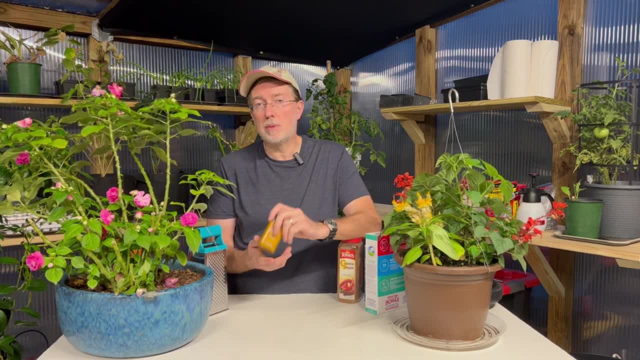 So it had no effect once they became used to the tumeric being on the potted plant And it just didn't do anything. as far as repellent it would, obviously it probably wouldn't have any effect to kill them, But as a repellent, no, it doesn't work for me. now the product. 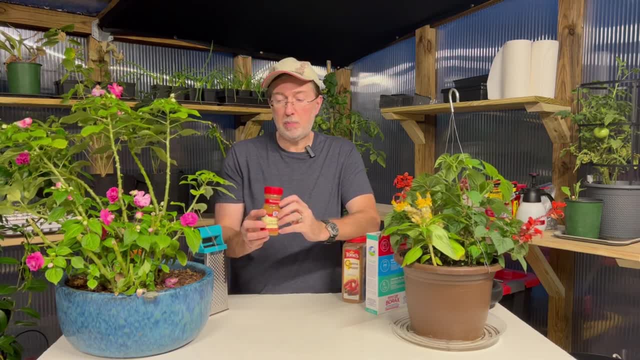 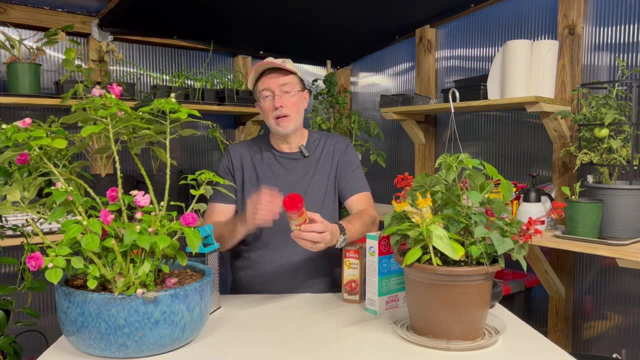 I have found a lot of success with when not killing ants, But repelling them from my potted plants is just common ground: cinnamon. Sprinkle it around the perimeter of the pot and it acts as a great repellent. It will keep the ants from going into the pot and establishing a nest. 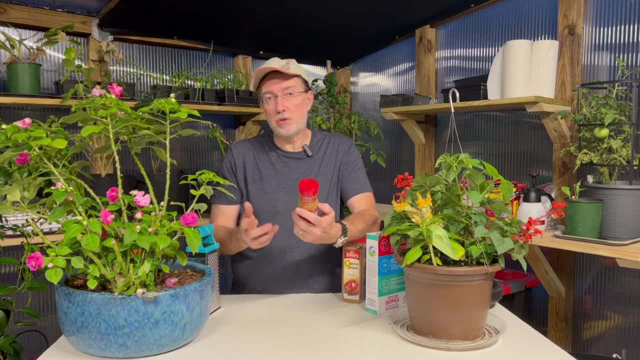 Even when it gets wet, as long as you've got a nice barrier on the edges. once it dries out It will retain that smell. probably having to do this, maybe once every three or four weeks in the summer, will act as a repellent for keeping those ants out of your potted plants. and 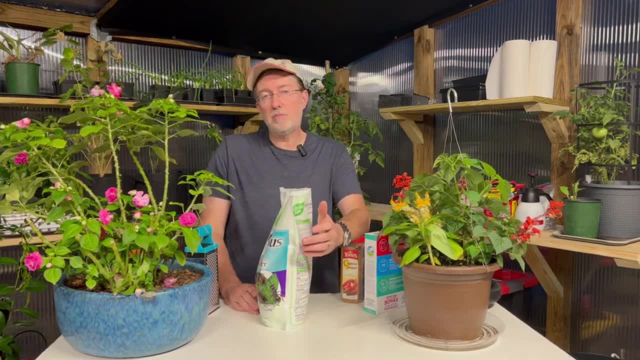 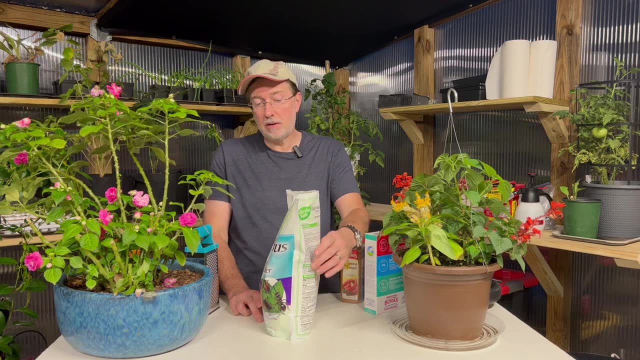 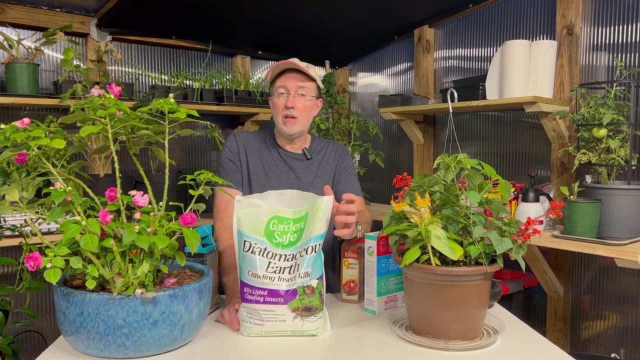 Ultimately into your living space now by far the most effective product I've ever found for controlling ants And your potted plants. that's not a pesticide, It's very safe, is diatomaceous earth, It's microscopic marine animals and it's in a very fine white powder when the ants come in contact with it. 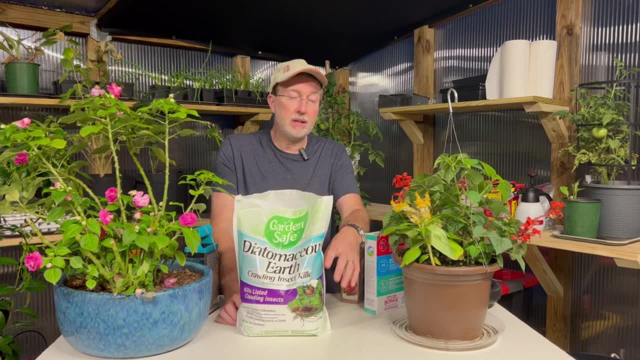 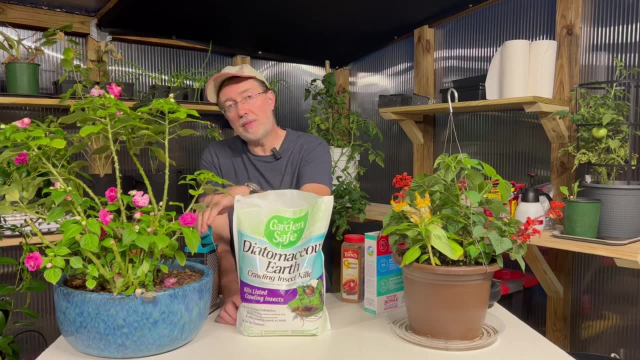 It will kill them. It won't kill them instantly, but they will die rather quickly and it will absolutely Prevent them from setting up a colony in your house plant. You'll just what you do. rather than making a ring around the edges of the plant, You just want to sprinkle it all over the soil. It's perfectly safe for the plant. 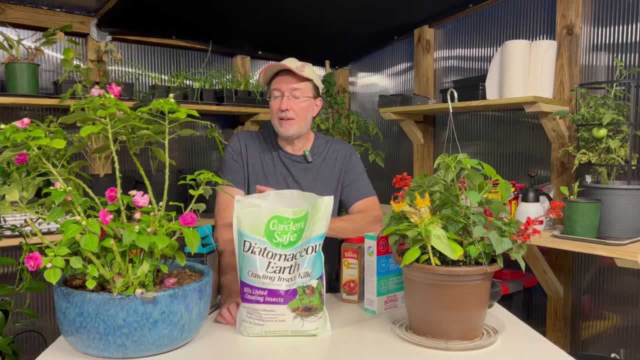 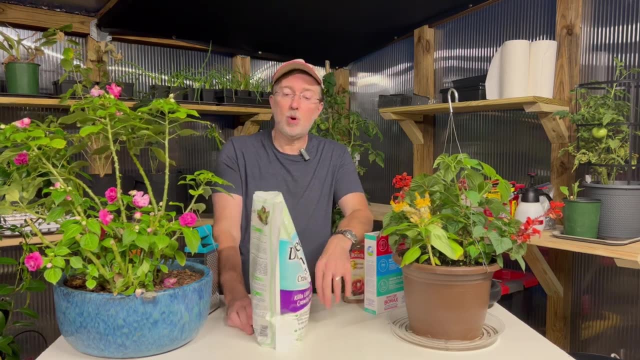 It won't affect it, It won't change the soil, and it's just the best thing I've found To stop ants from living in your potted plants. Now there's one thing I have to say about diatomaceous earth is, once it gets wet, it loses its effectiveness. 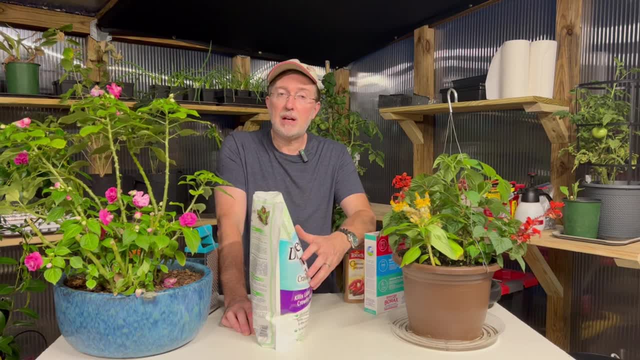 So watering- if you do a lot of watering in the summer, This could be something you're going to have to add a lot of during the summer months, But if you do it once a week, It will be act as a preventative and it will kill any ants that are in there at the time that you treat your your. 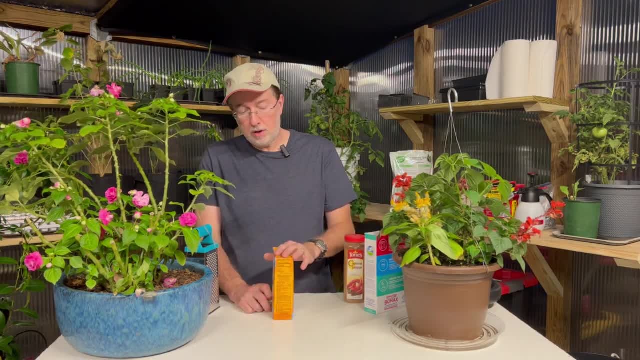 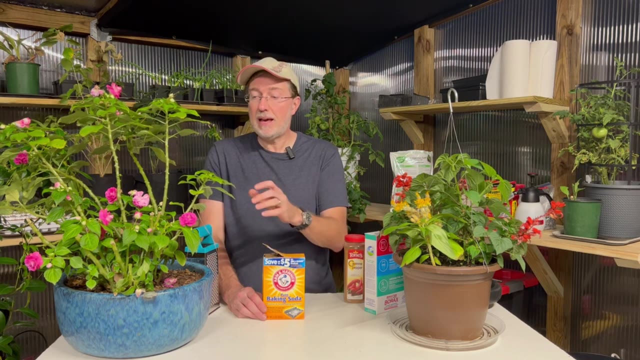 House plant or your outdoor plant. now a few extra products I wanted to talk about, because they're very commonly said to control ants in the garden is Baking soda, and although baking soda may kill ants when they ingest it, if they ingest it, The problem is the sodium portion of sodium bicarbonate can damage potted plants. 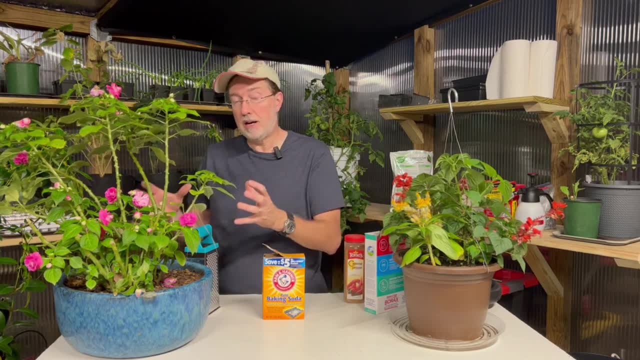 So if you're putting it in the garden, in an open area where you're not in a confined soil space And you may be a little bit more okay out there, But if you're talking about potted plants in that soil, You only have a limited amount of soil in the pot. It could very easily damage. the extra sodium could easily damage. 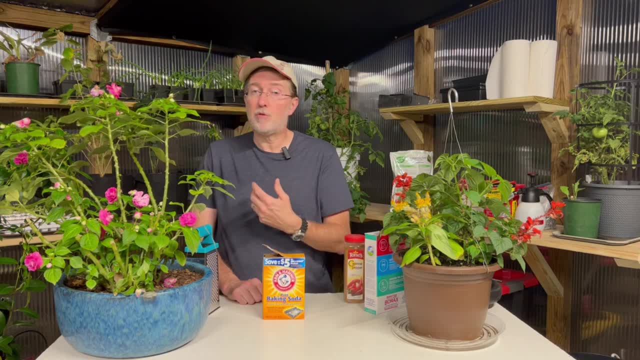 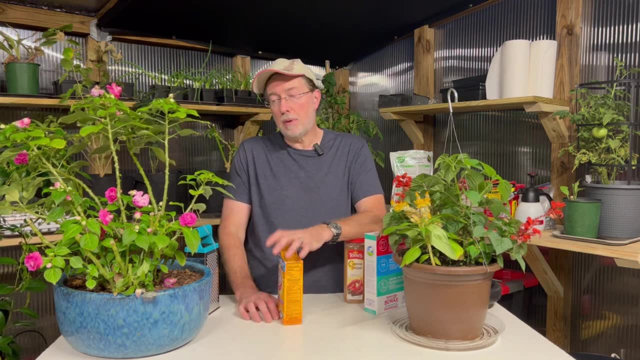 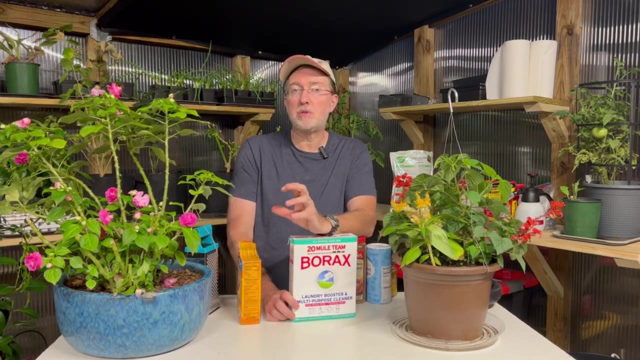 Your plant and also it may have a very limited effect on keeping ants out. Anyways, now, previously I had made a video about controlling ants in my vegetable garden, and that uses borax and Sugar, and that's a pretty common way to do it. It uses a special type of trap that you put it in and it's safe from the rain. 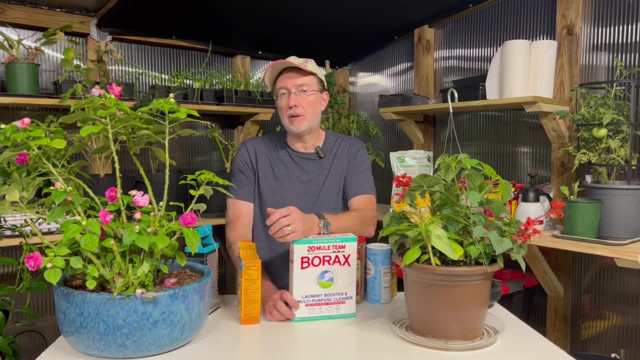 But I don't necessarily recommend for doing that in your potted plants. This is more of an open garden thing. I'll link the video up above for that as well, But I prefer the previous two That we talked about that were the most effective one: cinnamon for repelling and diatomaceous earth for killing. 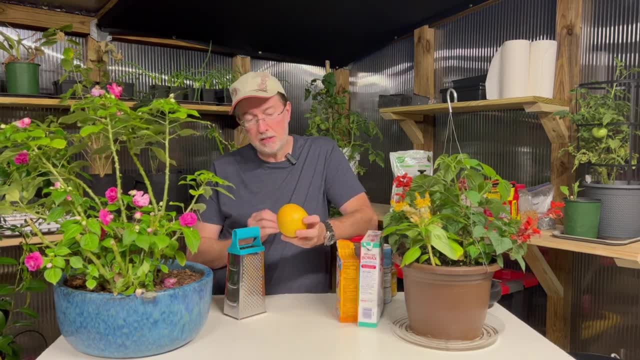 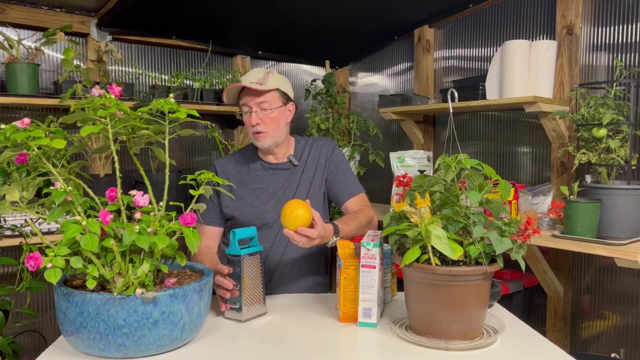 so another interesting way to Repel and possibly stop ants from getting into your house- plants as lemons, oranges and grapefruit- You can zest the outer skin and then sprinkle those Shavings around your plant, and some people say that that can actually interact with the ants nervous system. 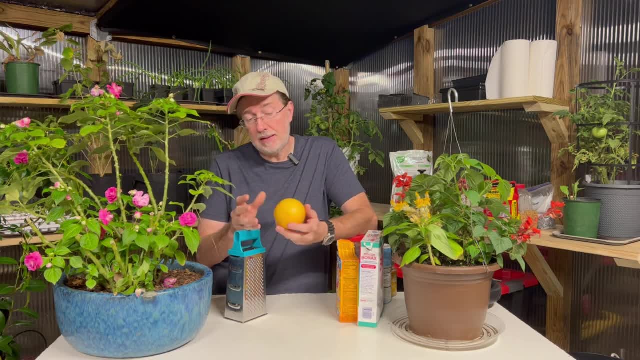 I don't know that for a fact, but it's an interesting idea. But, as I said, I like trying different things, especially if they're organic and there's no chance Of being contaminated with my plant or myself. So, guys, I just want to say thanks so much for watching. 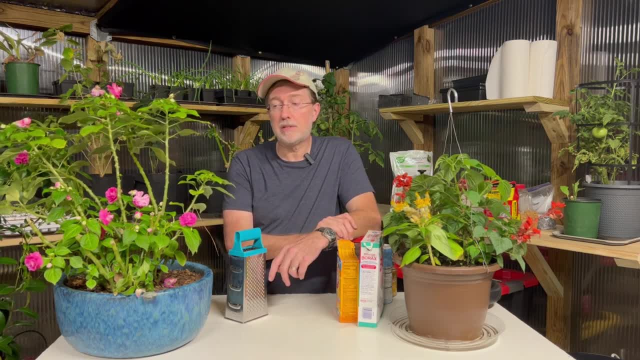 I really appreciate it and I hope you got something out of it. You did. I hope you'll like and subscribe and if ants are a big problem for you and you've tried something that really worked, I hope you'll leave something in the comments to let me know, because I'm always reading. 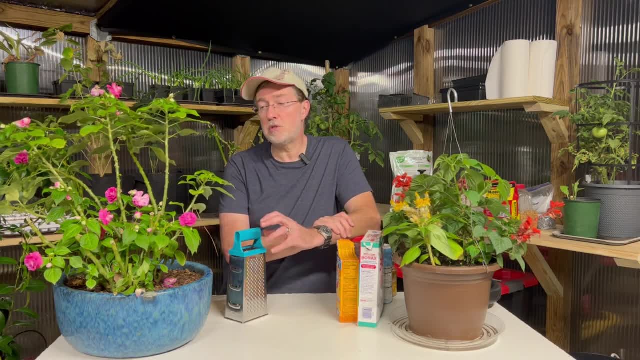 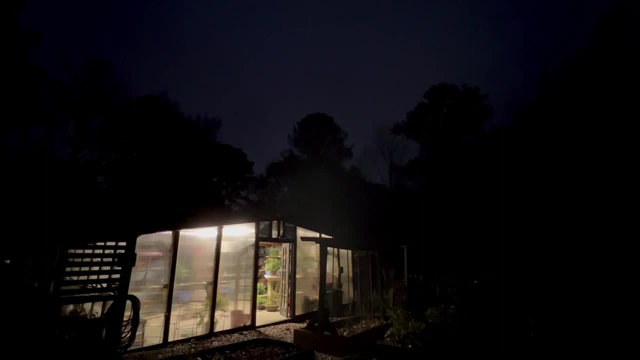 I'm always experimenting and I'm always wanting to learn new ways to do something safer and more effective than I do now. So have a great day, guys. You.